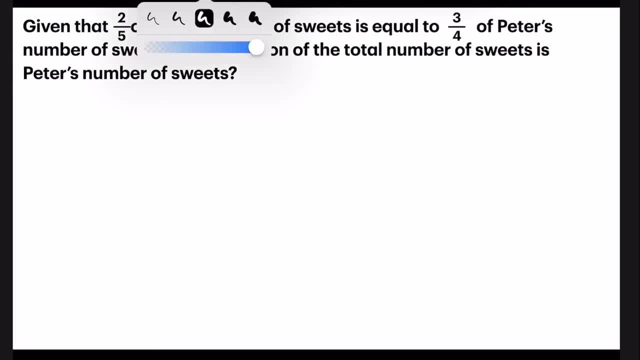 sentence and draw a model to show you what it means. So here we go, Jane and Peter. So 2 fifth of Jane's I'm gonna draw 2 fifth. okay, First of all, I just draw 2 units because that's the most important, part 2. 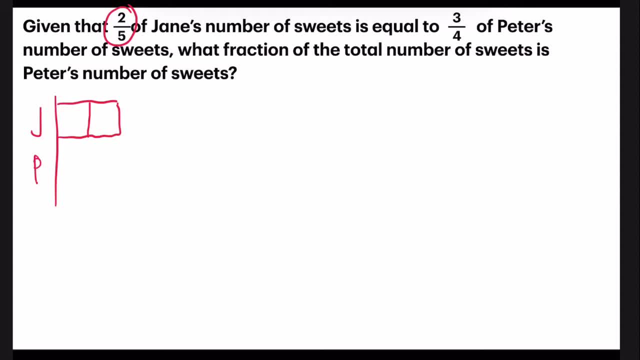 units of Jane is equals to 3 units of Peter's. So remember, bearing in mind it should be of the same length. So let me use a black color, okay, because they are saying that it's the same amount, But remember, for Peter it's cut into 3. 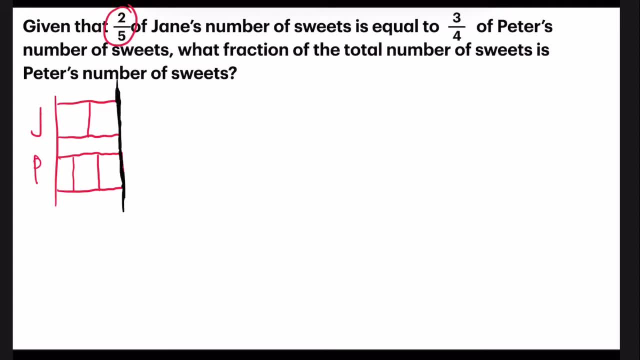 parts because it's three quarters of peter's. so now, having drawn the amount, that's equal. okay, the keyword equal, i am now going to draw the total number of sweets that jane and peter have. so, jane, if i have drawn two fifth, that means there will be three more units. 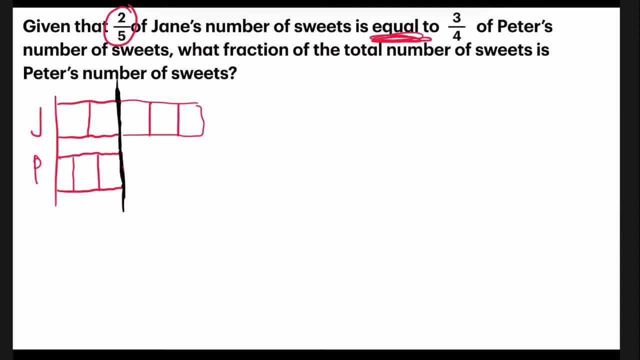 so let me draw three more units. okay, that's about the same size. and now let's go on to draw peter. since peter has already have three quarter drawn, that means there will be one quarter more of peter's. okay, now model drawn. do you observe anything in the model? 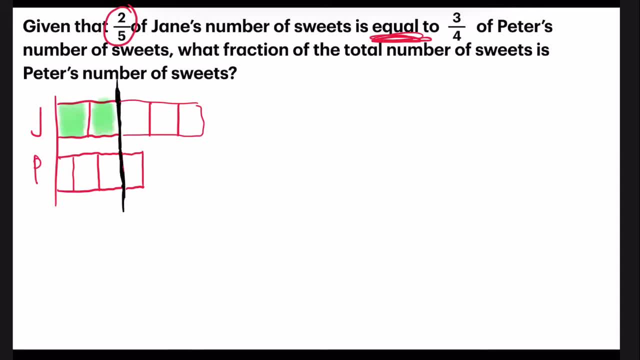 you see that- this part that i've highlighted in green- they are off the same portion, but every single piece is not cut up equally, so it's very hard to compare. so what do you think i should do now? since jane's has already drawn three quarters, that means there will be one quarter more of peter's. 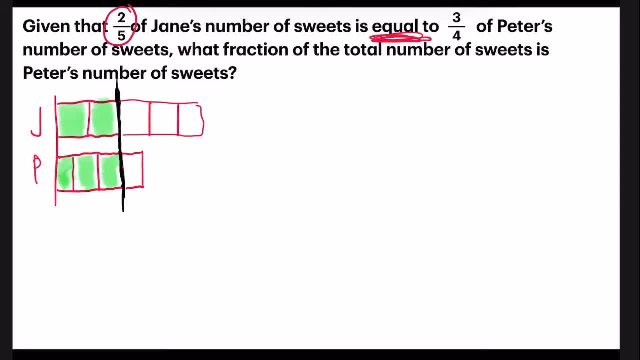 so jane has two units and peter has three. i will cut them into equal parts, two and three. i can cut them into six and six. so to cut jane into six parts, i need each unit to have three, and for peter to be able to have six parts i need to cut each unit into two. now you compare. 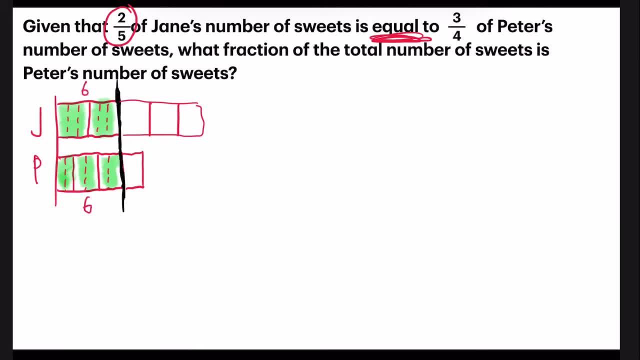 i have six on the top and six at the bottom, so now it is very, very convenient for me to compare. but as i have cut the model into three for jane, i should also do the same for the rest of the model. so if you count the total parts, 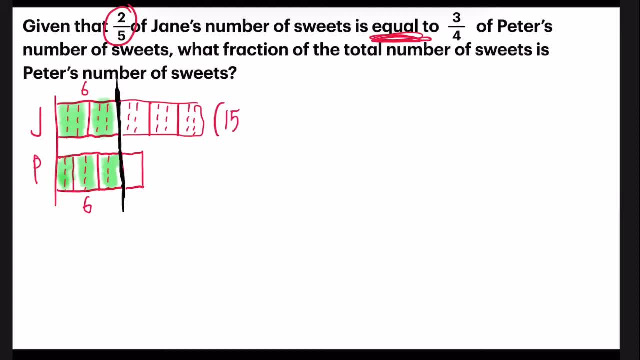 three times five, there will be 15 units in total for jane and for peter. i cut the rest as well into two. i should have eight units in all. so now we are ready to answer the question: what fraction of the total number of sweets is peter's? okay, so, peter, he has eight units in all and i have to find the. 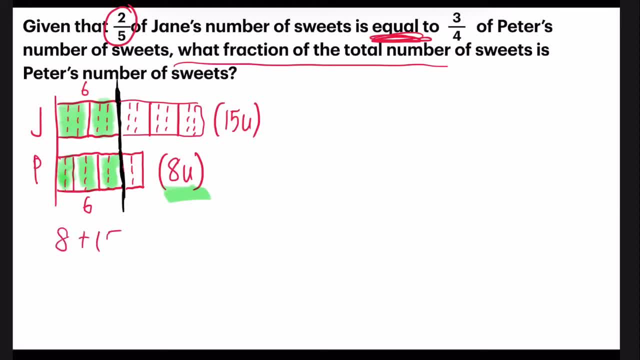 total, which is 8 plus 15, i will get 23.. so the fraction to my answer is 8 out of 23. that is my answer. okay, now we shall move on to using the method of same numerator. i'm going to write this out: 2, 5 of j. 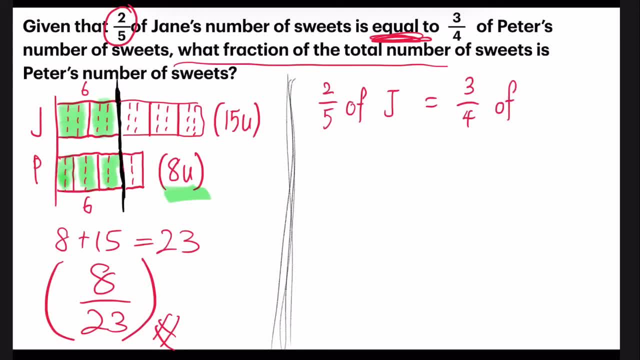 is equals to 3 quarter of peter. and observe this: two units is supposed to be the same. that's why the equal sign is there. so same thing. i'm gonna cut it into equal parts. that's why i will have to change the numerator into a number that's of the same, which is why i will multiply this type by 3, and for peter i have to. 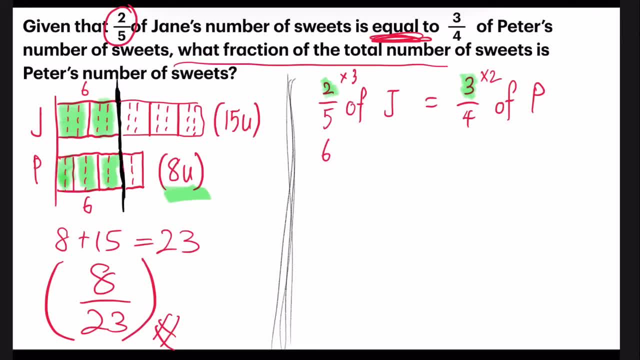 multiply by 2.. so my new fraction will be: 6 out of 15 of jane is equals to 6 out of 8 of peter. all right, at this point in time, the most crucial moment to link it to what we have done before, take a look at the 15.. 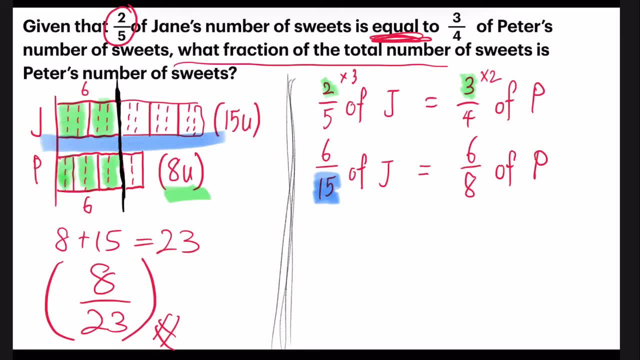 it is the same as the 15 units that we have drawn just now. and take a look at 8. it is also the 8 units that we have drawn up just now. so, if you recall, why do we have to change them into same numerator of 6 and 6? we are trying to make them into equal parts, like we have done just now. 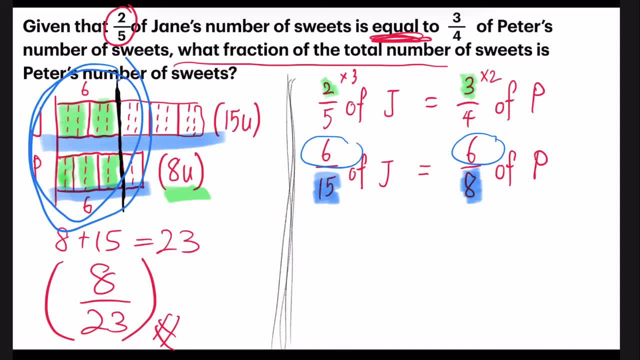 for our model drawing. that's the reason why we are changing it to the same numerator, And the denominator is the total units that Jane and Peter have. Take a look and now you can compare and see the idea. When you change it into the same numerator, what does it mean?